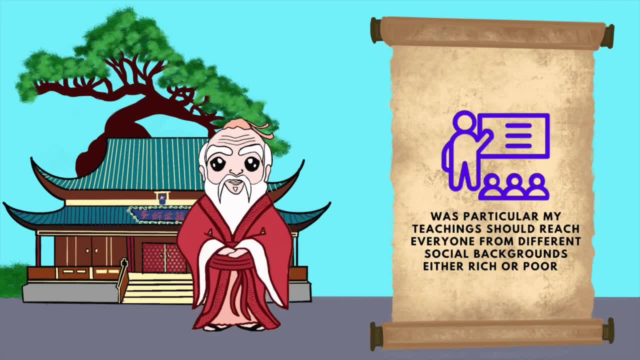 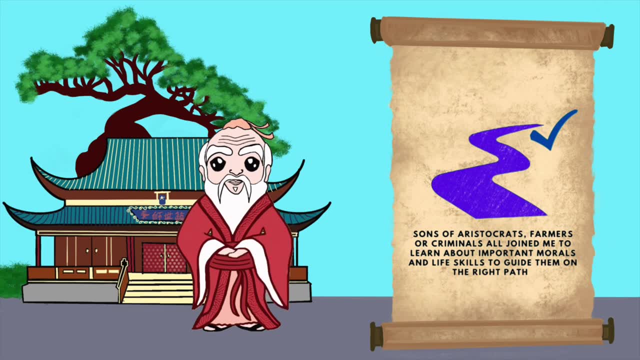 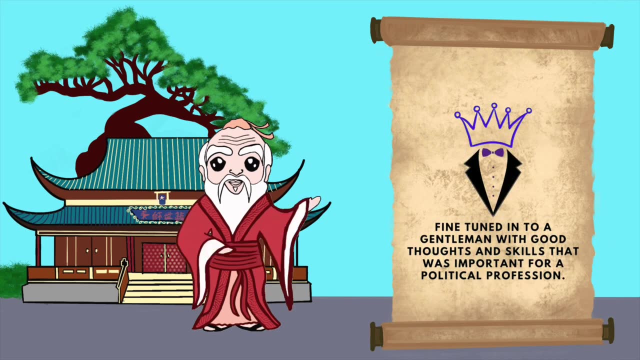 I repented from all social backgrounds, whether rich or poor. So sons of aristocrats, farmers or criminals all joined me to learn about important morals and life skills to guide them on the right path in life. I was happy they acquired the right morals and ethics and got fine-tuned into a gentleman with good thoughts and skills. that was important for a political profession. 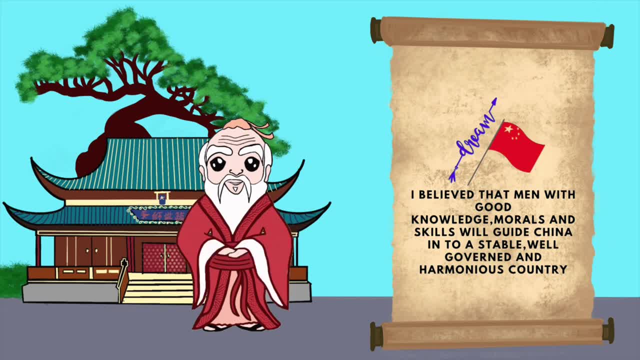 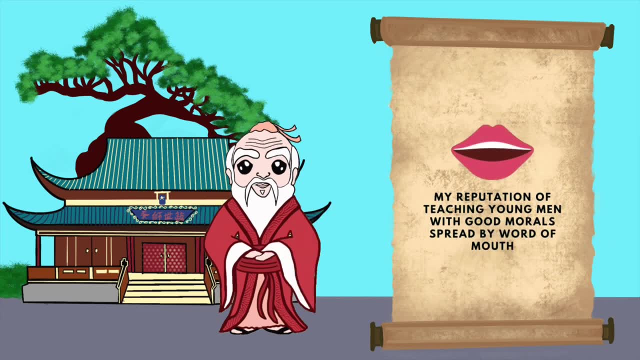 I believed that men with good knowledge, morals and skills will guide China into a stable, well-governed and harmonious country country. My philosophies and reputation of teaching young men with good morals spread by word of mouth. Hence I was approached for a high post of state's elder, where I advised on many 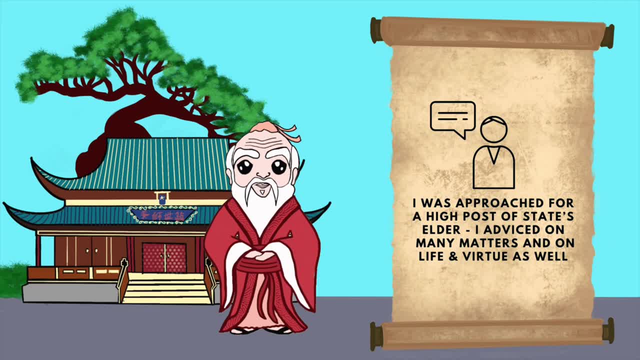 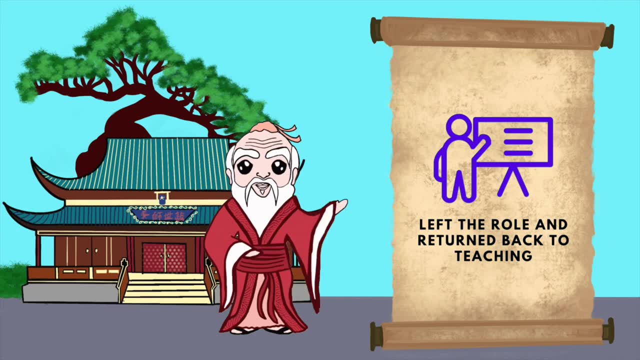 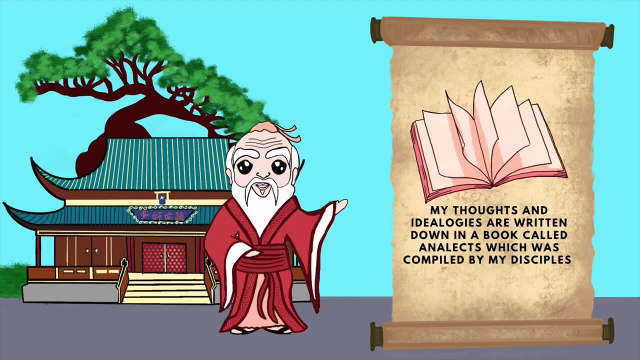 matters and on life and virtue as well. Over time I left the role and returned to teaching as I felt there were many distractions and deviations from governing well at that time. I later passed away in 479 BCE, and my ideas and philosophies spread throughout Asia. After my death, my thoughts and 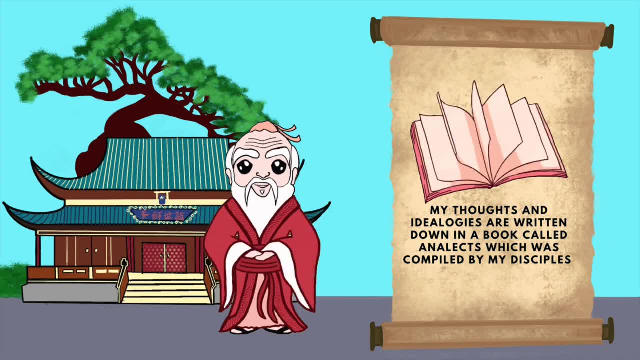 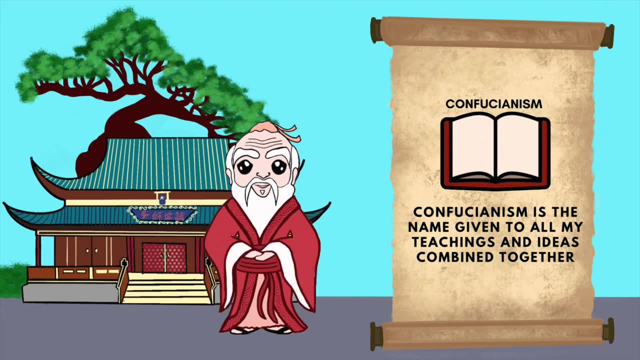 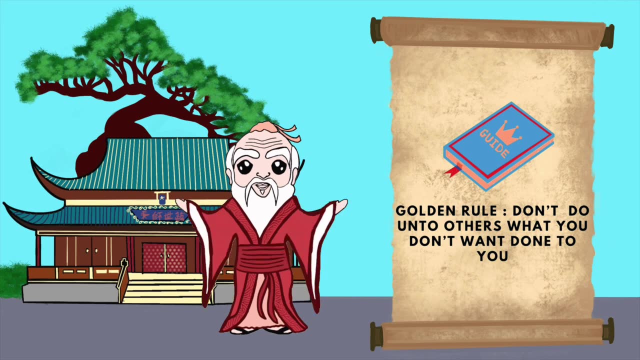 ideologies were written down in a book called Analects, which was compiled by my disciples. It was then that Confucianism was the name given to all my teachings and ideas combined together. My favorite golden rule was: don't do unto others what you don't want done to you. That means don't. 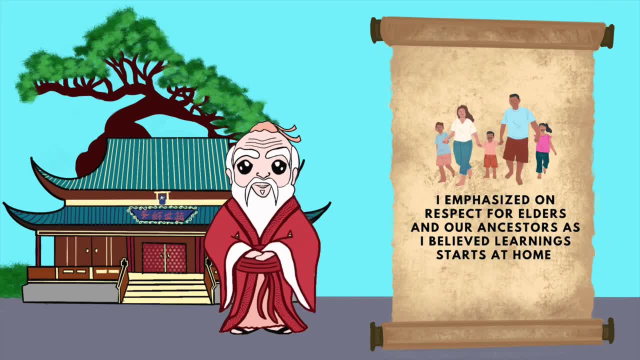 treat others in the way that you don't want to be treated. In my teachings, I emphasized on respect for elders and our ancestors. as I believed, learnings always start at home. In 1867, my teachings were translated to English by James Lake. My thoughts also. 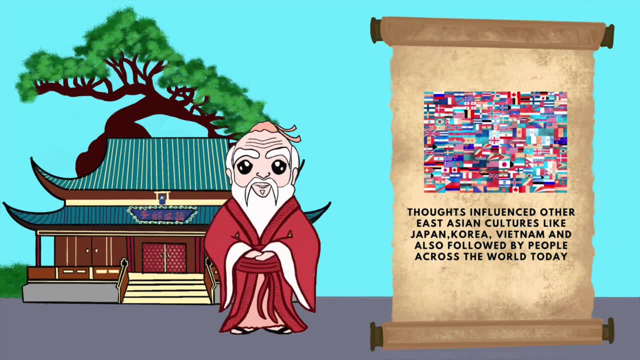 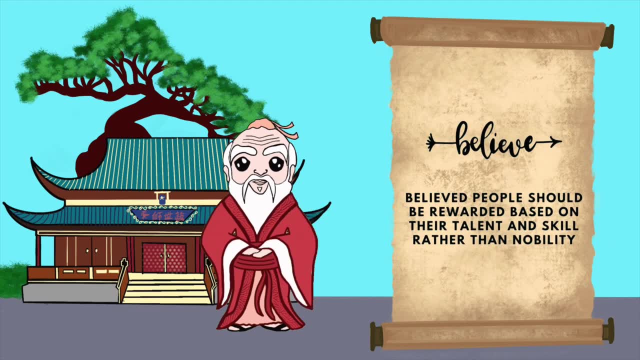 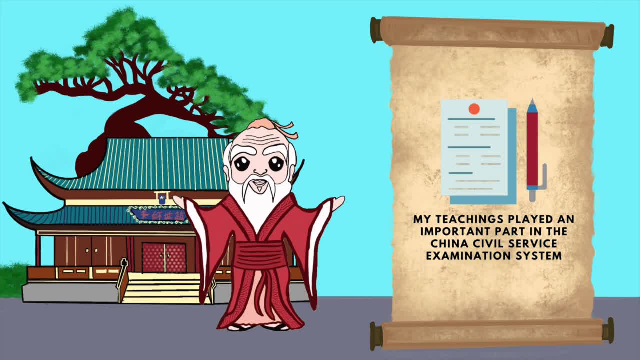 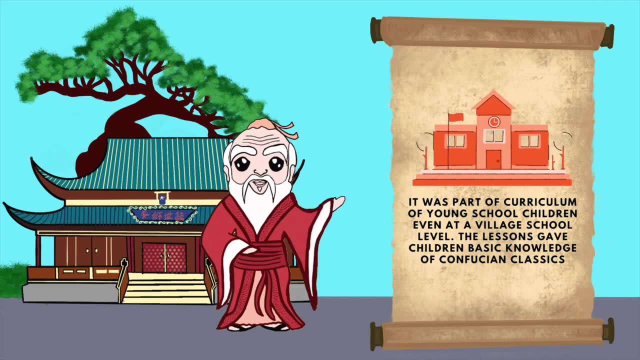 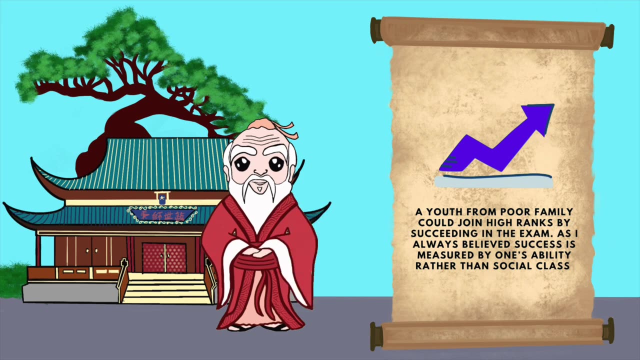 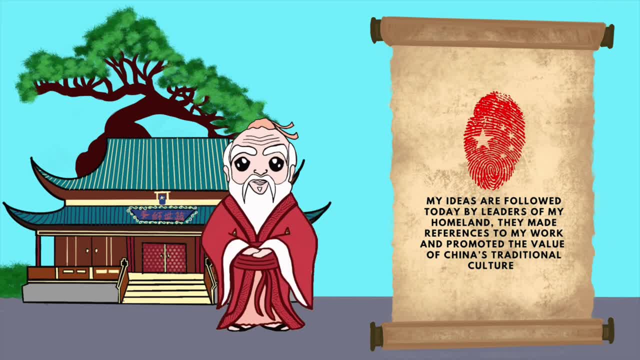 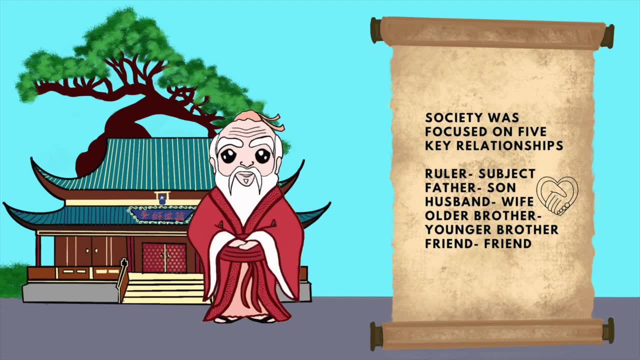 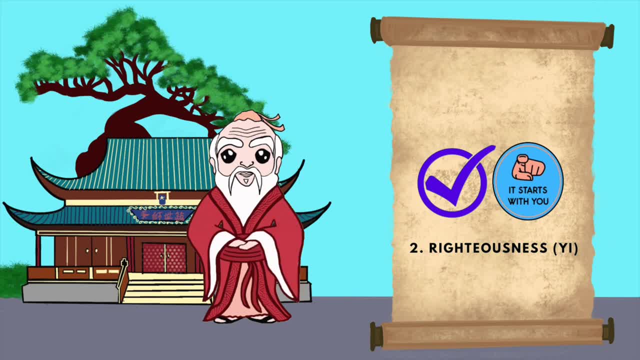 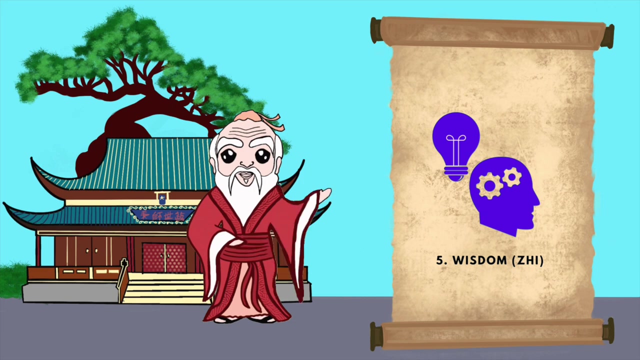 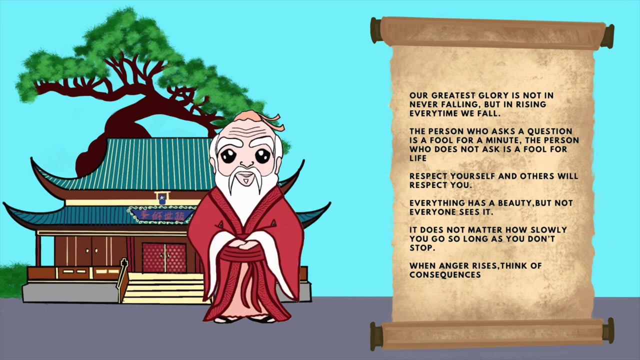 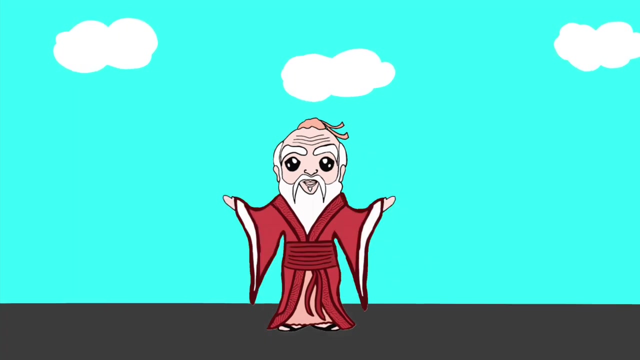